plus 4 plus negative 3.. So 5x- 4x, you have to combine them. It's just x equals negative 2 plus 4 plus 5x 4x. So 5x- 4x, you have to combine them. It's just X equals negative 2 plus 4 plus negative 3.. 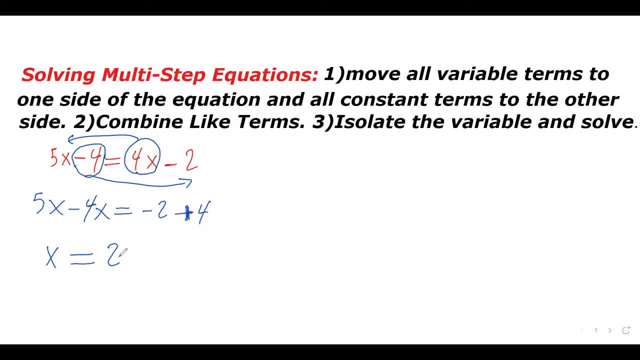 That's just positive two. So step number two is done And the last step we have to isolate which is already isolated: x. So this is our answer: x equals two. That's our answer. So here's two more examples. 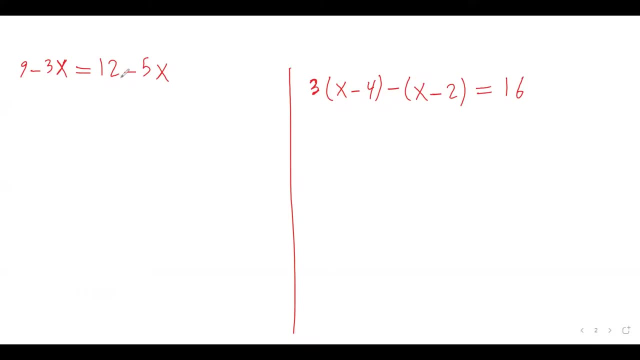 Here is the next one: Nine minus three x equals 12 minus five x. Again, the first thing we need to do is to move all the variable terms to one side and all the constant terms to the other side. So I have negative three x here. 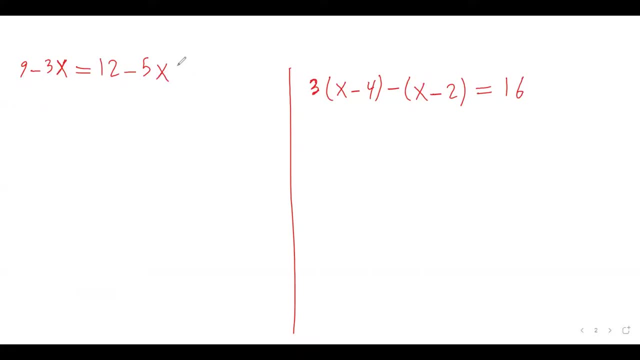 I have negative five x on the right side. I wanna move this negative five x to the left side. Let's do that. And then I wanna move this constant term to the other side. So on the left side I have negative three x. 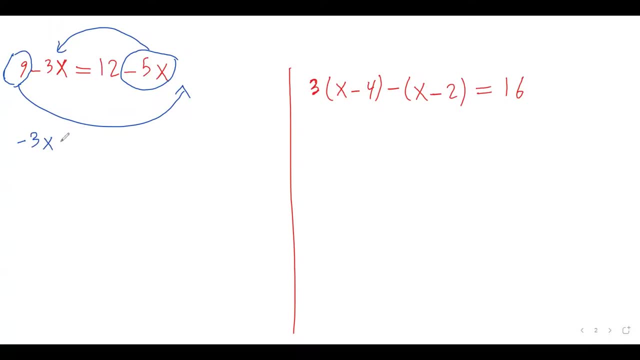 If I move negative five x from right side to left side, it becomes positive five x. This is my left side equals On right side. I have this constant term, I write it down: 12.. And then I'm gonna move this nine. 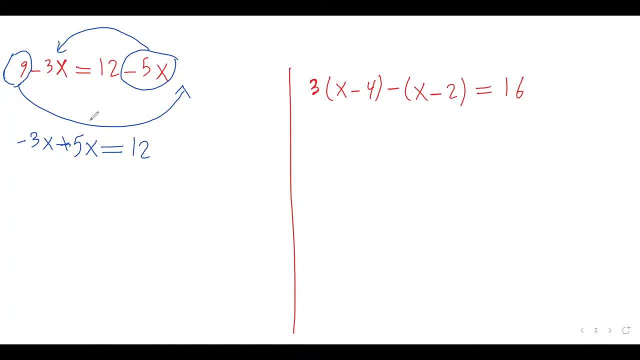 to the right side of the equation, It's positive nine. If I move it to the right side, it becomes negative nine. And now we have to combine like terms. I have negative three x plus five x, That is just positive two x on the left. 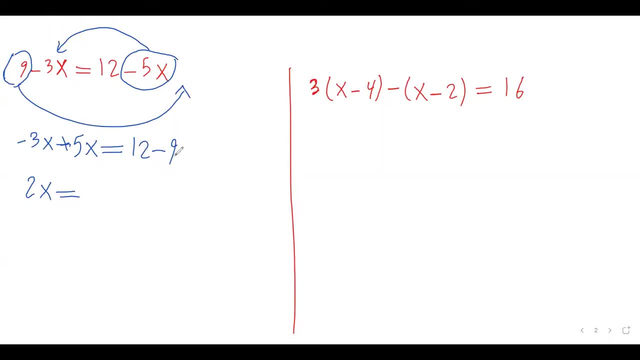 equals. on the right side of the equation I have 12 minus nine, which is three. So two x equals three, And now it's the number three. I have to isolate x. How can I do that? The x has a coefficient of two. 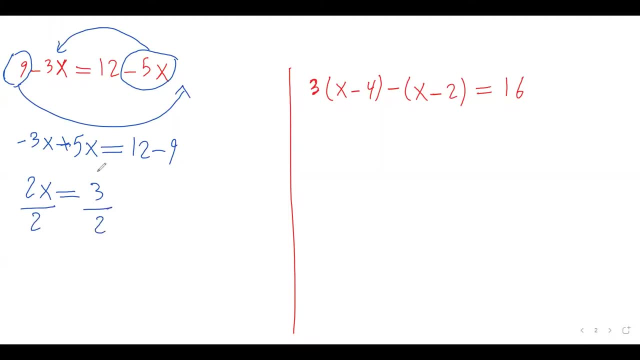 so I can divide both sides by two. So this two cancels this two. So we have x isolated by itself on left side equals three over two. This is our answer. All right, How about this set of equations? We have brackets: three x minus four. 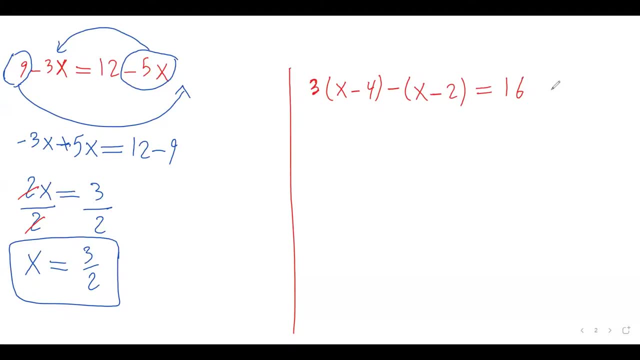 minus x, minus three, Minus two equals 16.. So when you have brackets in an equation, the first thing we need to do is to get rid of those brackets by. we can get rid of those brackets using distributive property. So if I can distribute this three into this bracket, 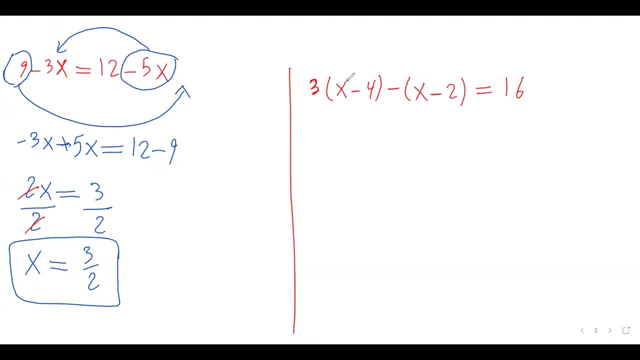 and that negative into this bracket so I can get rid of the brackets. So let's do that. I have to distribute this into this bracket. So three times x And then three times negative four And then we have to distribute this negative. 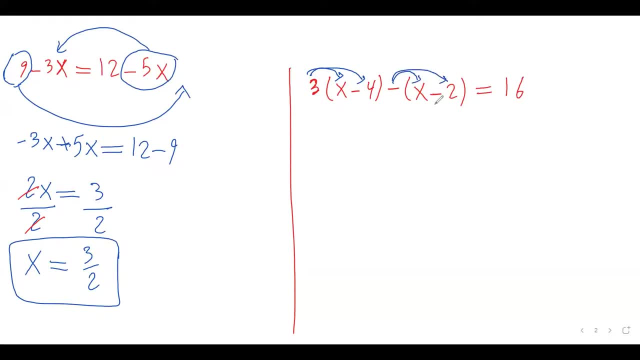 into this bracket as well, The first time and the second time. So let's write that down. Three times x is just three x. Three times negative four, that's negative 12.. Minus times x is minus x. Negative times a negative two, that's positive two. 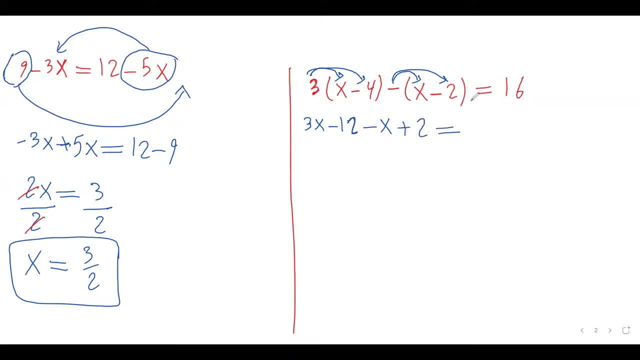 So plus two, These all are on the left side. This is the left side of the equation, And on the right side we have 16.. So now we got rid of the brackets, So we can follow those three steps. now We have to move all the variable terms to one side. 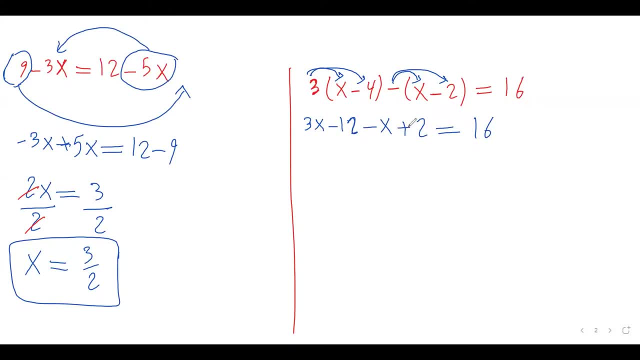 and all the constant to the other side. So on the left side I already have my variable terms, Just write them down. I have three x and then I have minus x. on the left side equals on the right side I have 16.. 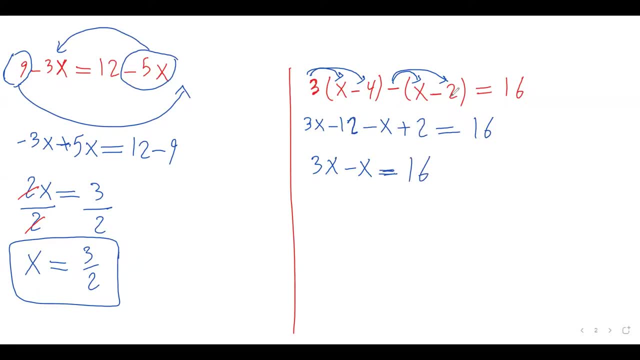 And I have to move all the variable terms to the left side. I have to move these two constant terms to the other side. So if I move this negative two to the other side, it becomes negative 12.. If I move it to the other side, it becomes positive 12.. 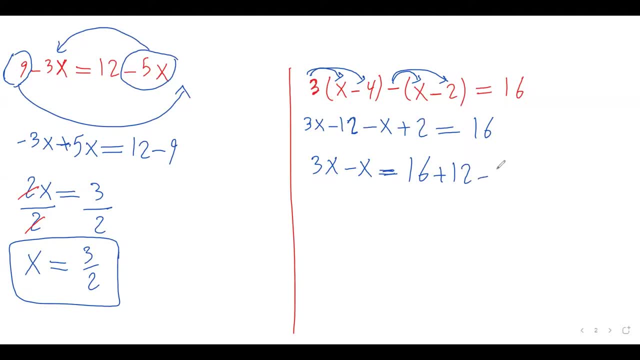 And I have positive two on the left side. I'm going to move it to the right side. It becomes negative two. And now we have to combine like terms: Three x minus x. that's just two x equals 16 plus 12 minus two. 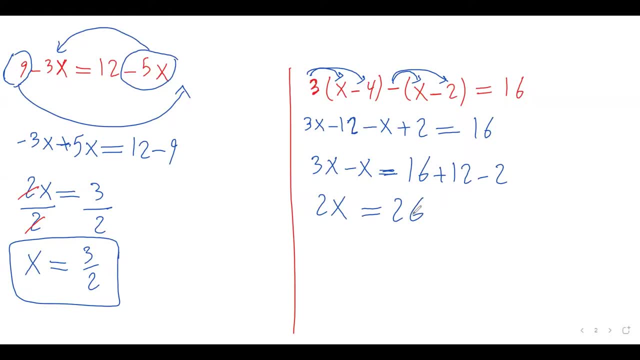 12 minus two is 10.. 10 plus 16,, that's 26.. So I have 2x equals 26.. I have to isolate x, so I have to divide by the coefficient, So 2x divided by 2, and we have to do the same thing to the right side as well. 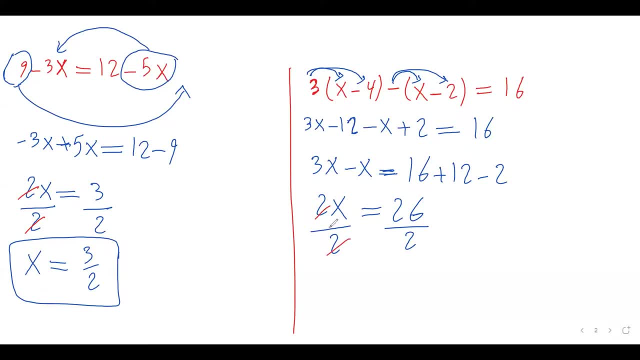 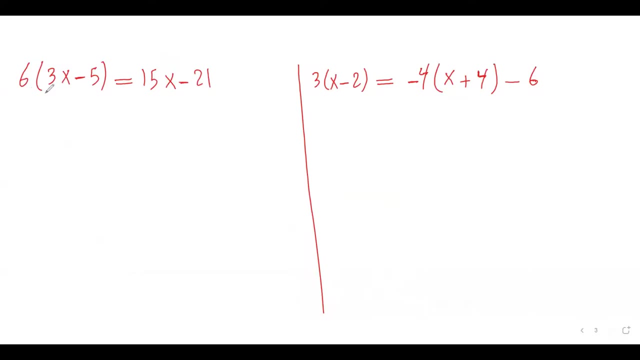 So this 2 cancels that 2.. I have x equals 26 divided by 2, which is 13.. This is our answer. Let's do two more examples. So here is this one: 6 bracket: 3x minus 5 equals 15x minus 21.. 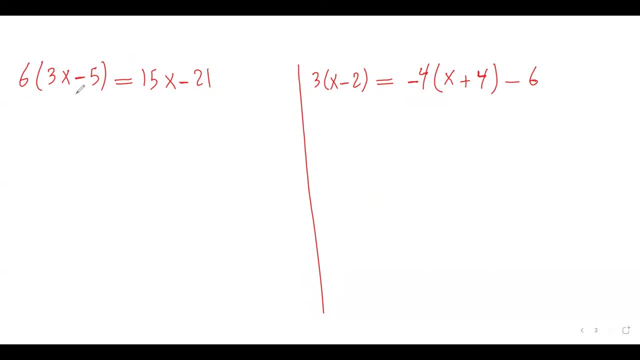 Again, we have bracket, so we have to get rid of that bracket by using distributive property. So let's distribute this into the bracket: 6 times 3x, that's 18x. 6 times negative 5, that's negative 30, equals 15x. 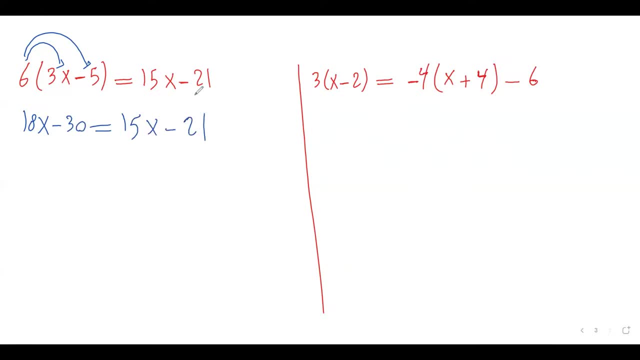 15x minus 21.. Now we have to move all the variable terms to one side and all the constant terms to the other side. I want to move this 15x to the left side, So I have 18x minus 15x equals. on the right side, I have negative 21,. 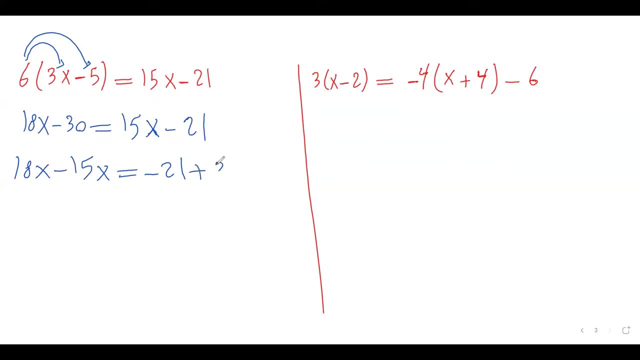 and I need to move this negative 30 to the right side. it becomes positive 30. So now we need to combine like terms: 18x minus 15x, That's just 3x, equals negative 21 plus 30. That's positive 9.. 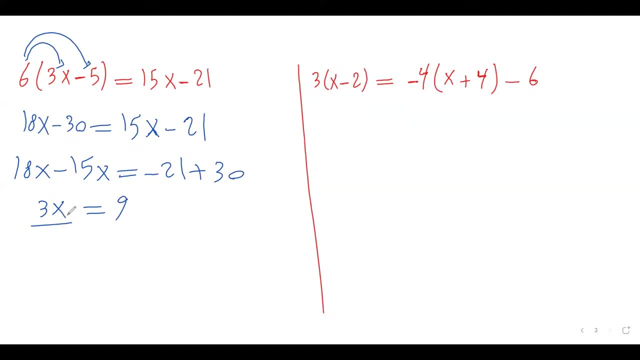 Then I have to isolate x. I need x by itself. So 3x divided by 3.. 9 divided by 3.. This 3 cancels this. I have x on the left side and on the right side, 9 over 3 is just 3.. This is our answer. 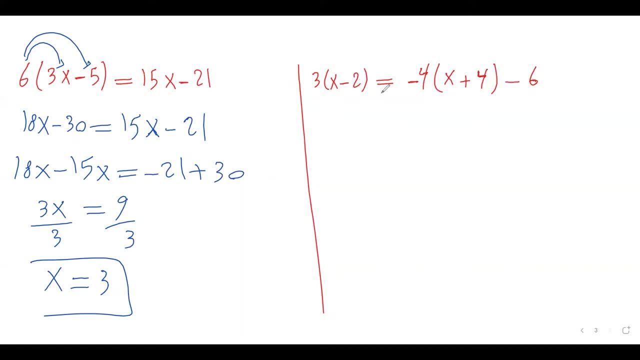 How about this one? 3 bracket x minus 2 equals negative 4 bracket x plus 4, minus 3.. That's negative 6.. Again, we have brackets. The first thing we need to do is to get rid of those brackets using distributive properties. 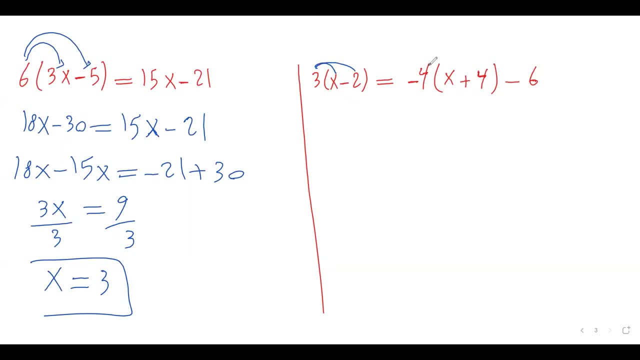 So I have to distribute this into this bracket and I have to distribute this negative 4 into this bracket. 3 times x is 3x. 3 times negative 2,, that's negative 6, equals negative 4 times x, that's negative 4x.